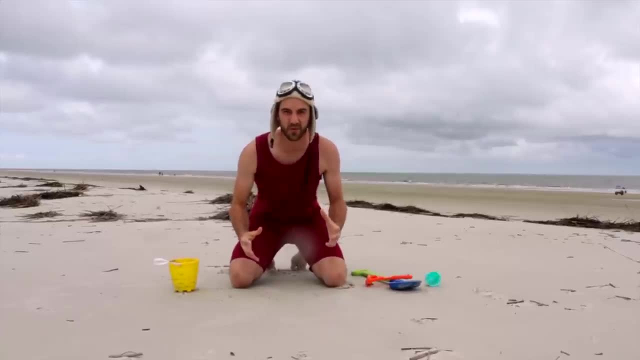 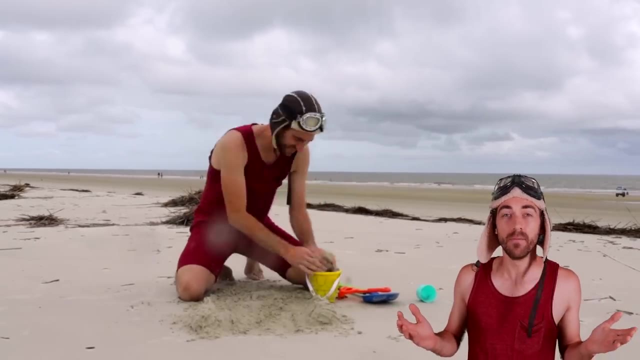 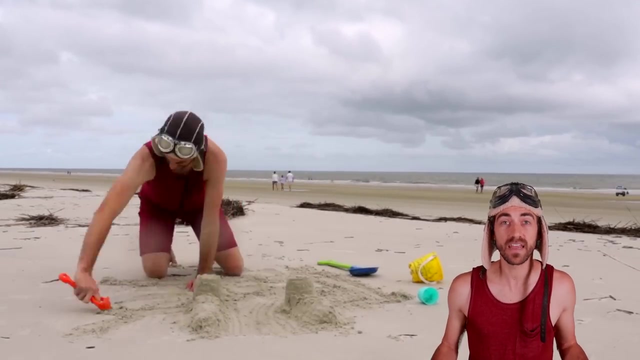 I'm going to do. I want it to be really big and really cool. I'm going to get started. Okay, So you can build your sand castle any way you want, but I like to follow three simple steps. The first step is drawing out the shape of your sand castle in the sand. 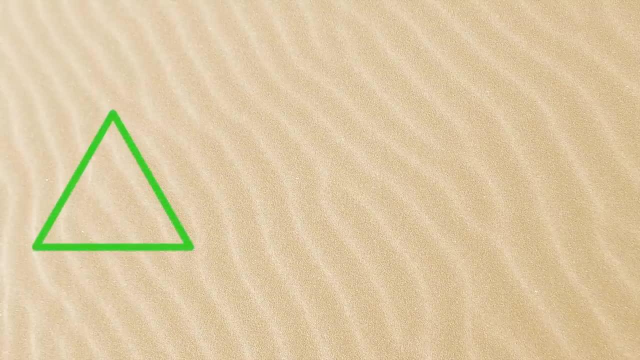 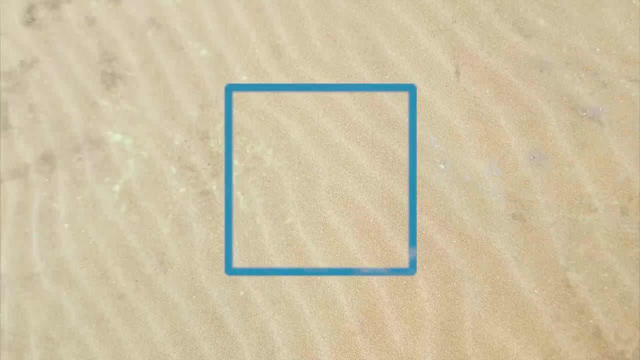 There's lots of different shapes. you can try like a triangle or a circle or even some kind of a crazy made-up shape, but I'm going to go with just a regular square. The second step is to build up a big pile of sand. This is going to help your sand castle. 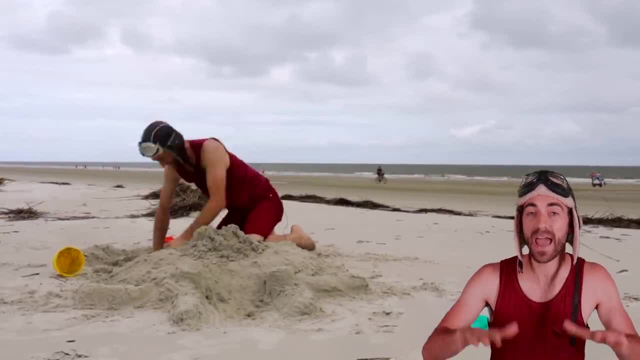 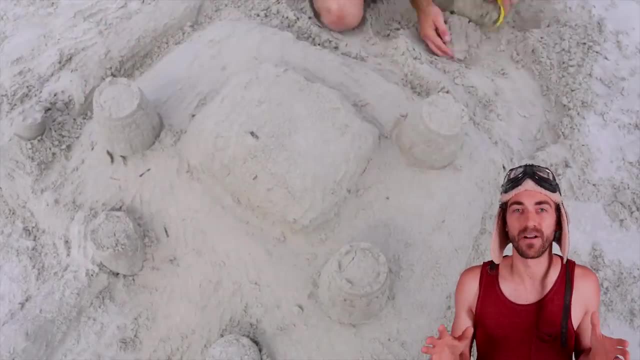 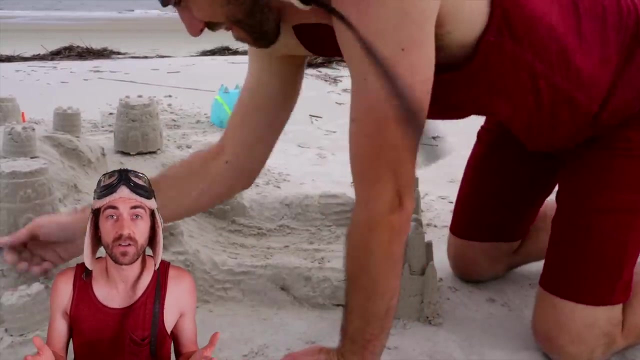 look really tall and really cool. Just make sure you pack it down really good before you put anything on top. The third step is the really fun part. This is where you start putting all the castles on top. You can also look around you for things like leaves and sticks that you can put on. 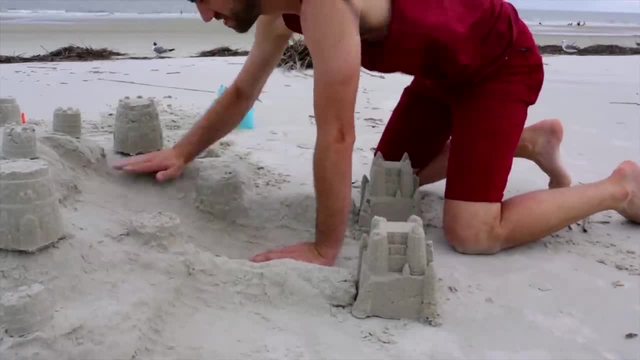 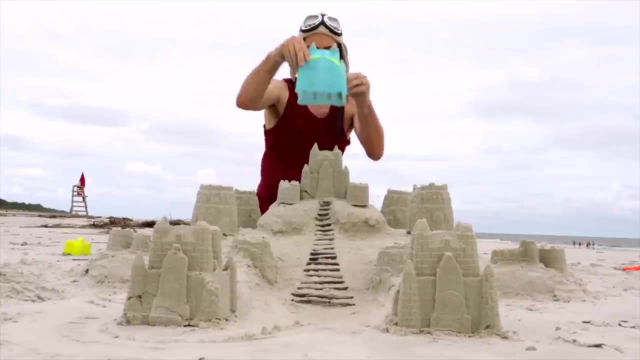 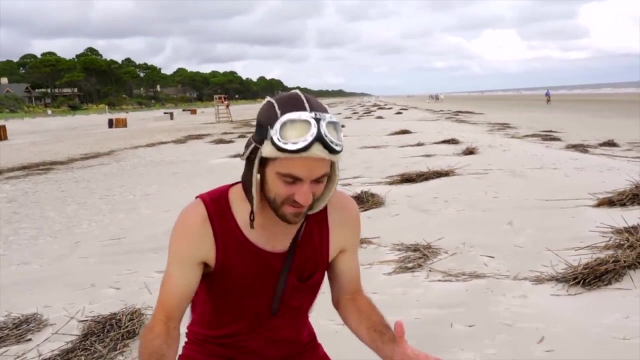 your castle to make it really cool too. All right, Here we go. All right, guys, I'm all done and I'm really excited. I'm excited with how this sand castle came together. Can I show you around a little bit? 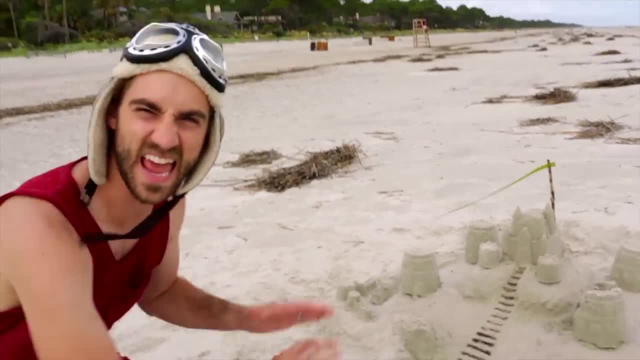 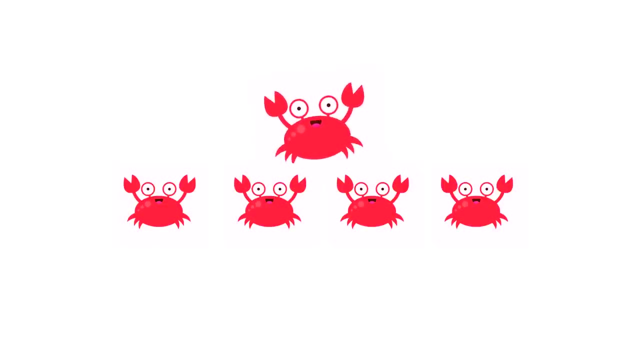 So the cool thing about sand castles is you can kind of pretend anybody lives here. So I pretended this was a crab kingdom, so lots of crabs were living in there. So the crabs would come up here in the beginning and they have to come past these two guard. 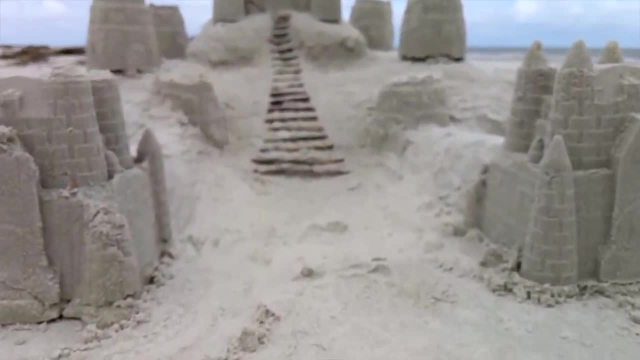 towers. These guys are making sure that no crabs are coming in here that aren't supposed to. So the crabs come in here, and then they see this big staircase in the middle of the sand castle. So I'm going to show you how this sand castle came together. 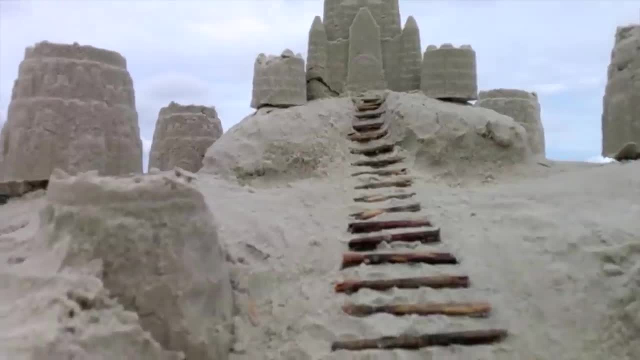 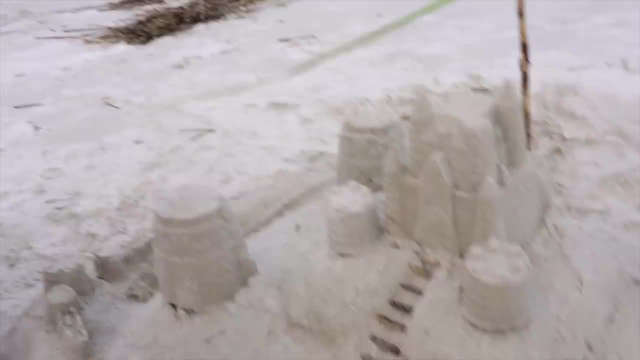 So the crabs would come up here in the beginning and they have to come past these two guard towers. The crabs go behind every wall and a multi-day process by their own. See what little biom備 you need. 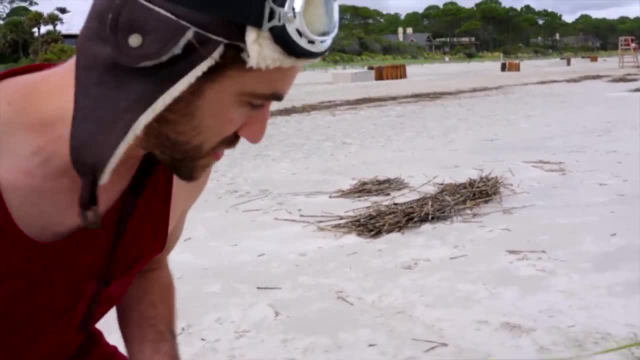 So it would be in the middle of the sand castle. See, if I set up a cold door, I'll know that really well, Awesome. No, this is external. Same here in the crew. Here they open the door and this is the big staircase up to the king crab. So they climb.